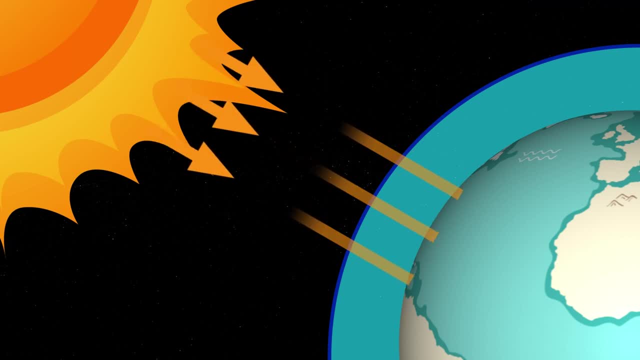 sends its rays to Earth, and our planet absorbs much of this energy, causing it to warm. In response, the Earth emits energy back into space in the form of a greenhouse effect, In the form of infrared radiation, or, more simply, heat, As this heat tries to escape. 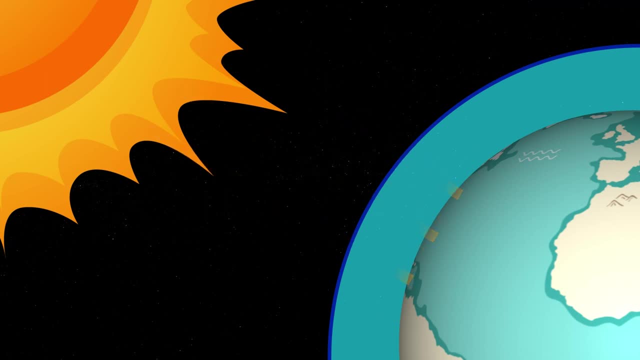 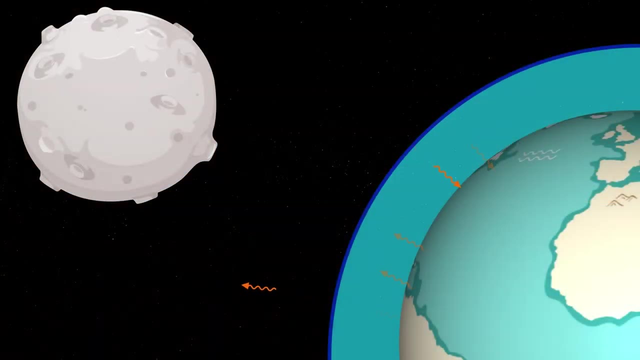 the atmosphere. certain gases present in our atmosphere, known as greenhouse gases, like carbon dioxide, methane and water vapor, capture and hold some of this heat. This trapped heat keeps the planet warmer than it would be without these gases, Without the greenhouse. effect, Earth's average temperature would be much colder, much colder than it would be without the greenhouse effect, making it a less hospitable and possibly impossible for life as we know it to exist. This process has been in play for billions of years, ensuring 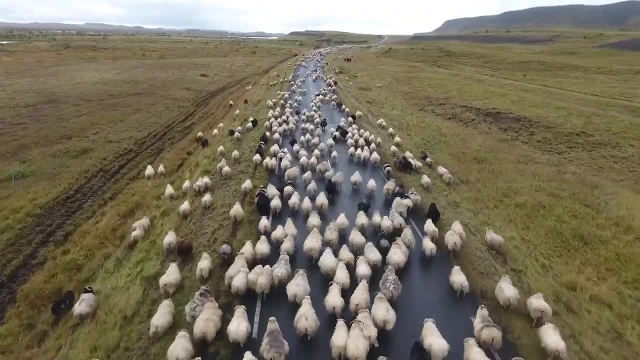 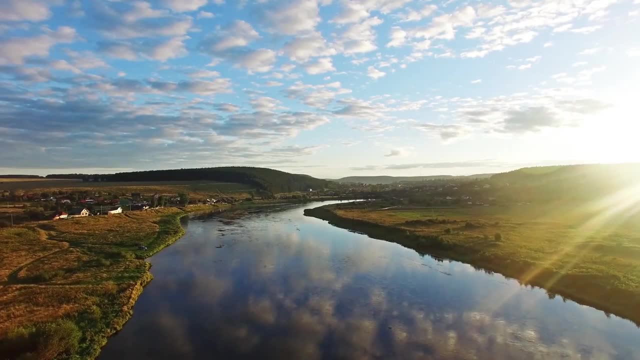 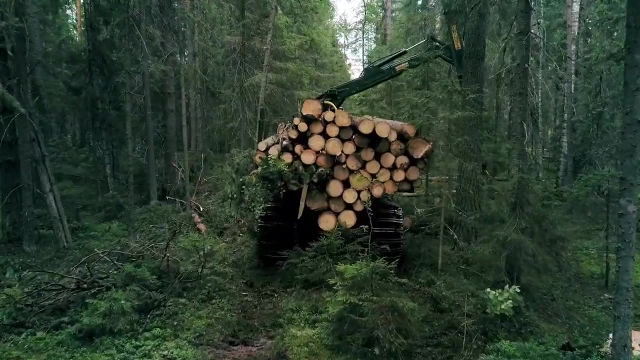 our planet remains within a temperature range suitable for the vast biodiversity, including us, to thrive. While the greenhouse effect is natural, human activities have been giving it a powerful boost, making that blanket around Earth thicker and trapping more heat than necessary. This is where things get problematic. 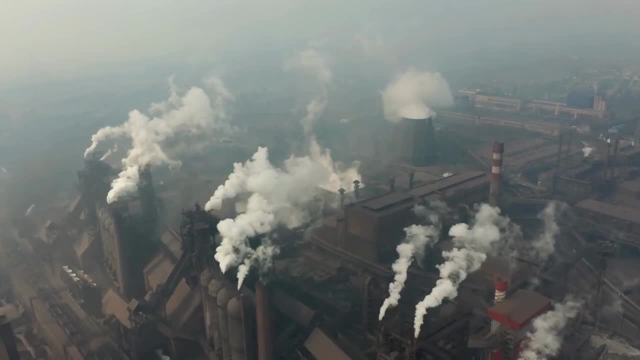 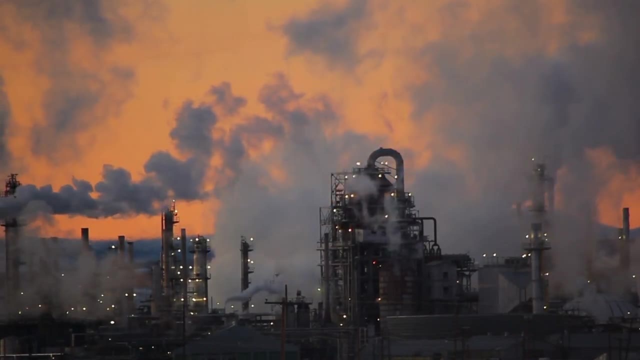 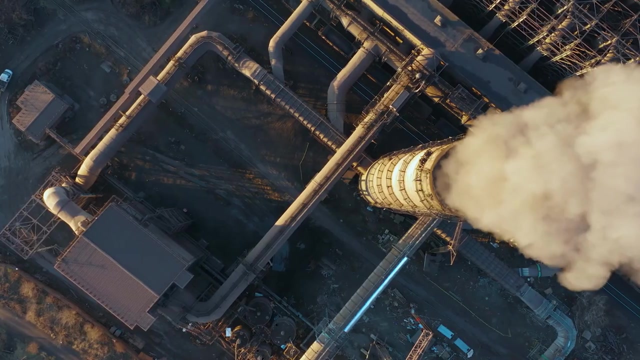 Burning fossil fuels. When we burn oil, coal and natural gas for energy, we release large amounts of carbon dioxide and other greenhouse gases into the atmosphere. Think of cars, factories and power plants. To operate, they often rely on the burning of fuels and in 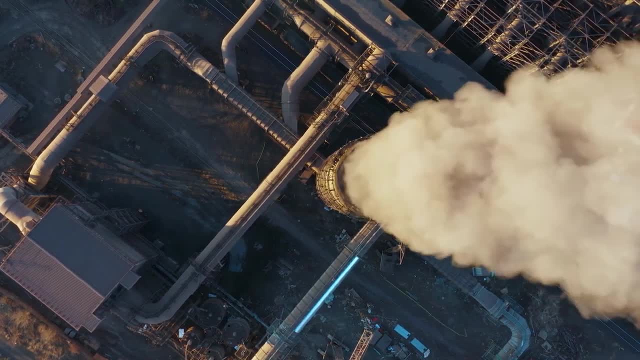 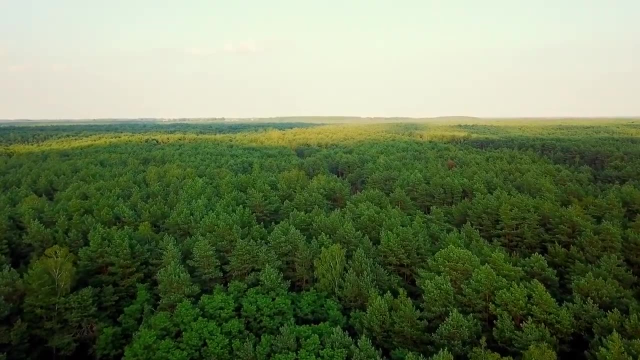 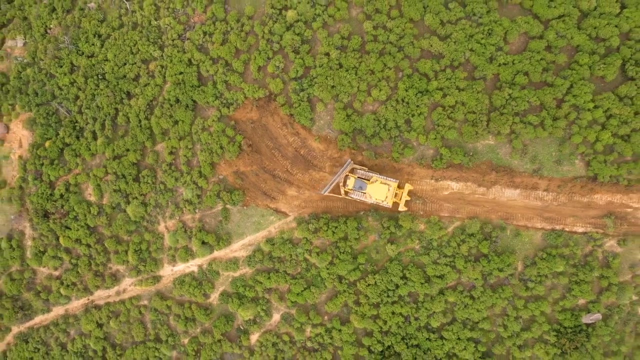 the process, contribute to the buildup of the greenhouse gases. Deforestation Trees act like the Earth's lungs, absorbing carbon dioxide and giving out oxygen. But when we cut down vast areas of forests for urban development or farming, we not only release the stored carbon dioxide in those trees, but also reduce the number of trees. 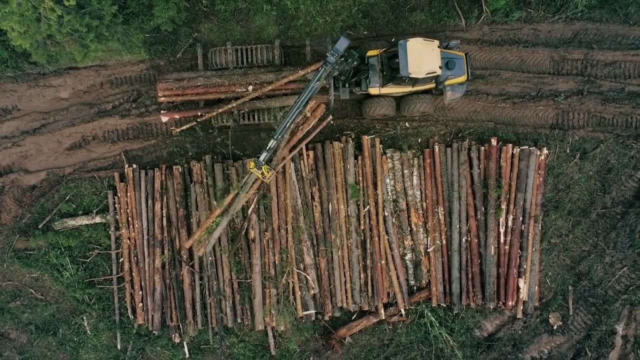 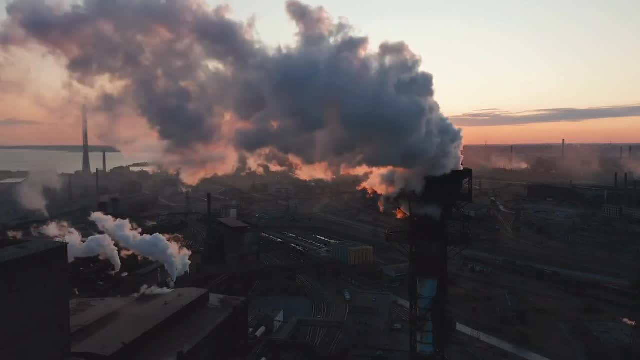 left to absorb future carbon dioxide in our atmosphere. Industrial activities and agriculture. Many factories release various greenhouse gases during production. Additionally, certain agricultural industries are also producing more and more greenhouse gases during production. For example, the greenhouse gas industry is producing more and more greenhouse gases during production. Additionally, certain agricultural 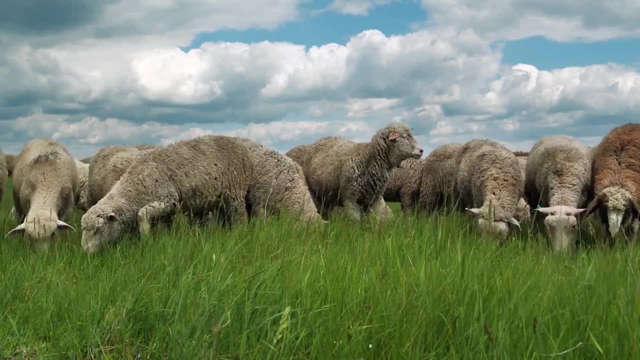 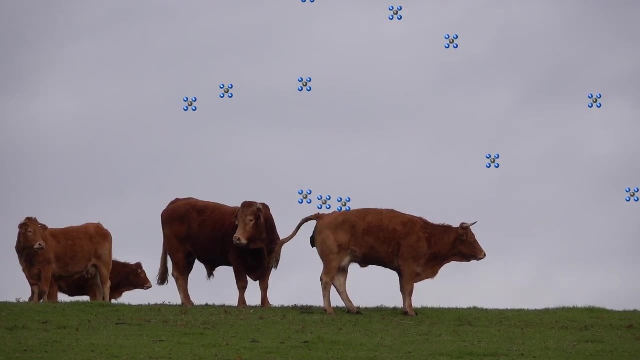 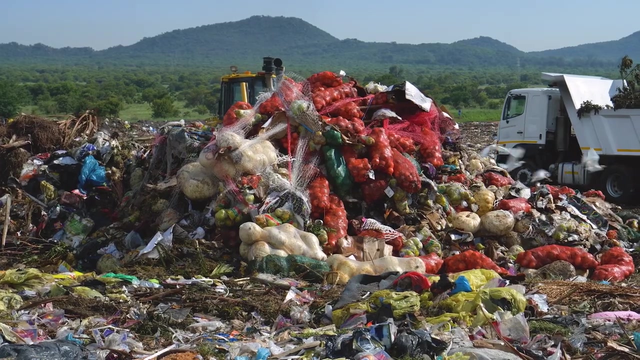 practices emit methane, a potent greenhouse gas. Cattle, for instance, produce methane during digestion. Yup, cow burps are an issue too. Waste management- Landfills full of organic waste release methane as the waste decomposes. Improper waste management intensifies this problem. 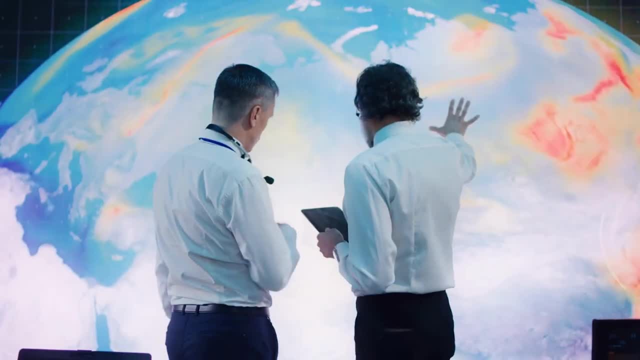 As humans amplify the greenhouse effect, Earth's average temperature rises, leading to what we now commonly refer to as轉 News. Mother North lives a lot less compared to her country left in the middle of a select group, so more, but about 3 timesAM.